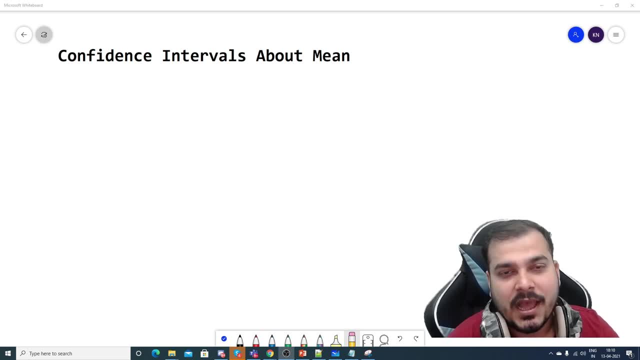 You know. so we'll try to discuss what exactly is confidence intervals and why it is actually important And and a lot of things that we are going to see, And we'll try to also solve that specific problem that was given in the interview. So, to begin with, what we are going to do, guys just understand what exactly is confidence interval. In order to understand this, first of all we need to understand what is point estimate. So I'm just going to write it down. So, point estimate, So suppose how, how, if you really want to 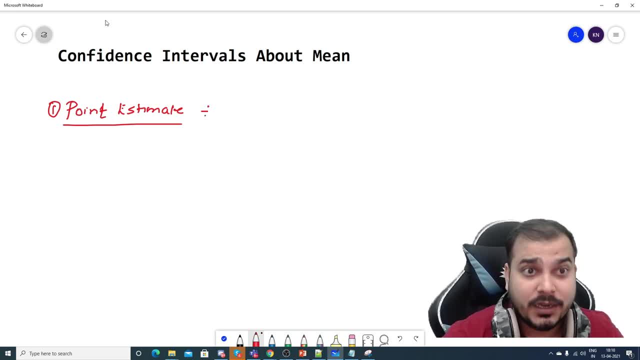 understand about point estimate, and this point estimate is important in order to find out the confidence interval. Now, usually in most of the experiment guys, just imagine that you will not be knowing the population mean, because it will be very difficult to just know the population mean altogether because population size is usually huge. But with respect to that, we may be able to find out the sample mean because if we consider some sample values from that specific population, we will be able to get the sample value which we represent. 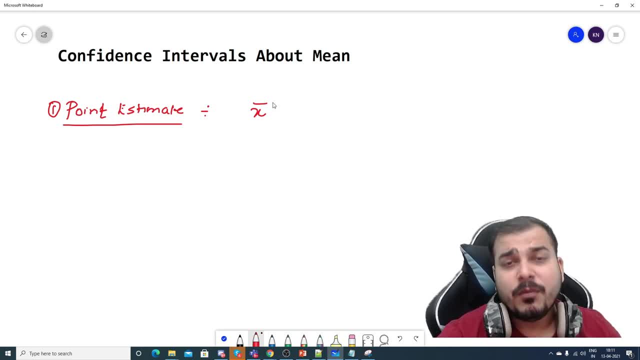 it as x bar. Now, with the help of this x bar, we'll try to estimate the parameter of the population mean. right Now, in this particular scenario, we see, x bar is nothing but it is the point estimate. Okay, so this exactly is the point estimate to basically calculate the parameter, that is, your population mean. And obviously we know that in based on the central limit theorem. you know, if we take multiple samples and if we try to basically create the sample mean, it can. 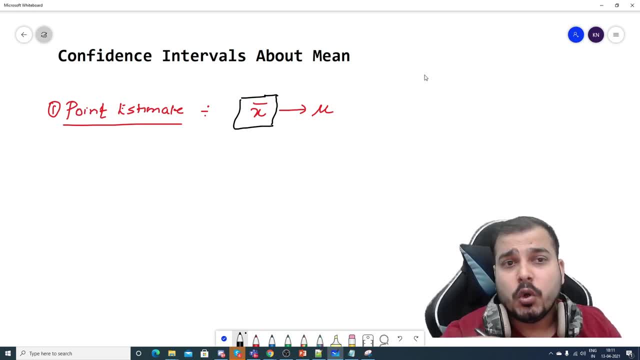 be approximately equal to the population mean you know. so this is exactly the point: estimate. And what does confidence interval basically say? that by considering this particular sample mean and with some confidence intervals like 95%- suppose I'm taking an example of some confidence interval of 95, 95%- I will be able to find out the range of the population mean, probably from what limit to what limit it may fall on, So it may have a lower limit. 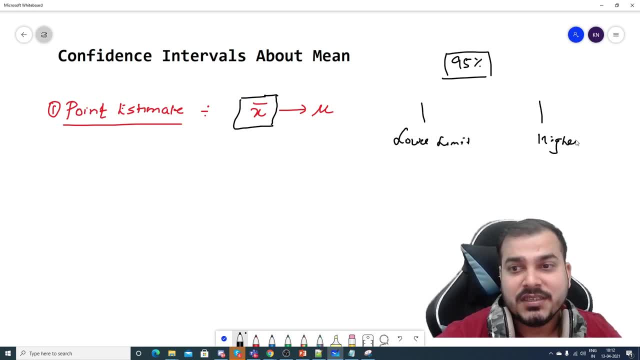 and it may have a higher limit. So this is basically my range that I that I can get with respect to the population mean, and this particular range may be 95% confidence interval. So this is the entire 95% confidence interval, right? So if I, if I try to draw this in the form of a graph, okay, so usually we know that most of our distribution follows this kind of Gaussian distribution. And if I take this to this, the tail region, which is the extreme region and probably 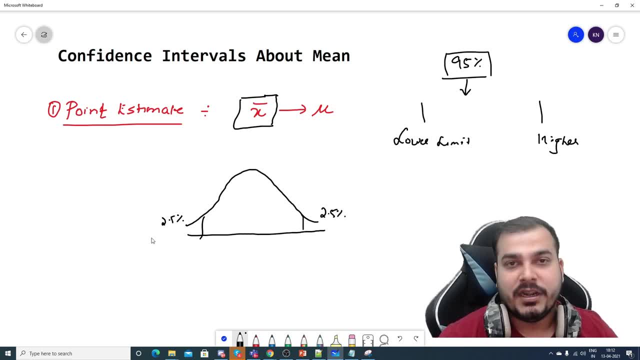 this is my 2.5 percent of data, and 2.5 percent of data. if my problem statement says that i have to find out with respect to the 95 percentage of confidence interval, then that basically means i need to find out the region from this place to this place. this will be my lower limit and this 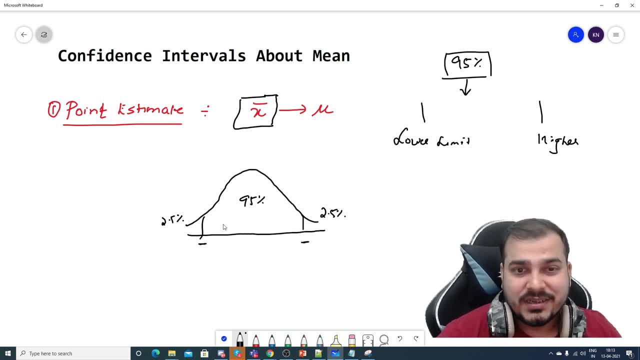 will basically be my higher limit. okay, now, with respect to this, uh, we'll try to solve this particular problem. and uh, in order to solve this particular problem, again, guys, there are two ways. the first way is, basically, if you are given population standard deviation and if you are 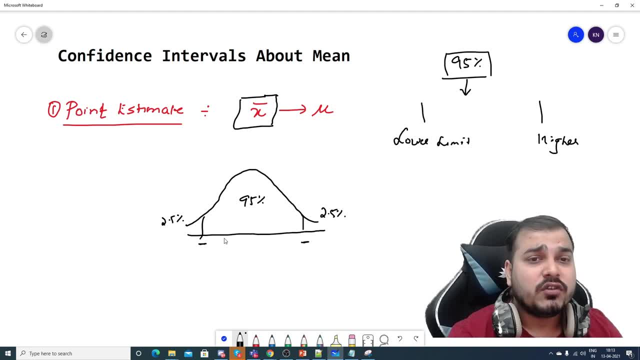 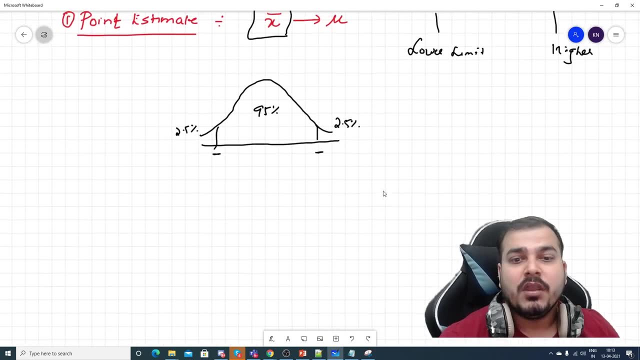 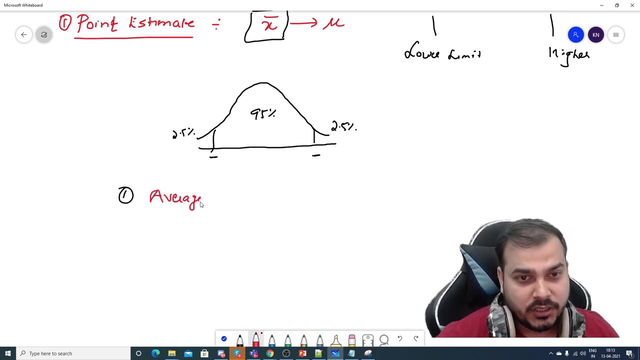 not given population standard division in this particular example. we'll try to solve this particular problem. statement: if you are given a population standard deviation. so let me just repeat the question that was asked in the interview. so the in in the interview it was said that please find out the average, the average mean, or i can just write average size. 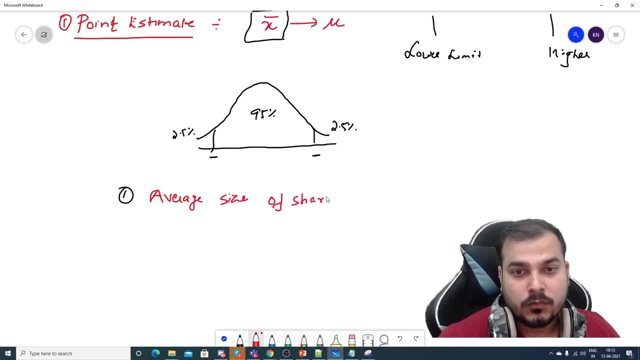 size of sharks, sharks in the sea. okay, so this is the problem statement that was given to the interviewer, to the um person who was actually attending the interview, and they told them that they can actually use whatever techniques, whatever they know- you know, they can make any kind of assumptions- to solve this particular problem. now, how to answer this kind of question? 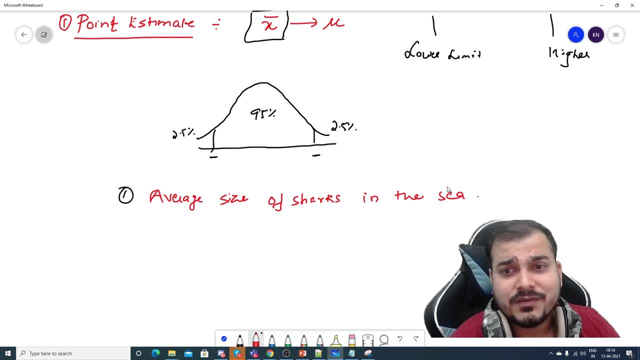 guys, because if someone says, okay, how to find out the average size of the shark in the sea, you'll be thinking how to find out the average size of the shark in the sea. you'll be thinking about various ways. the best, there are different, different ways, guys. one can be done with the. 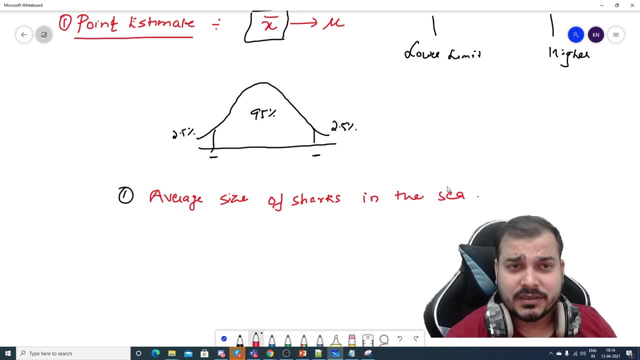 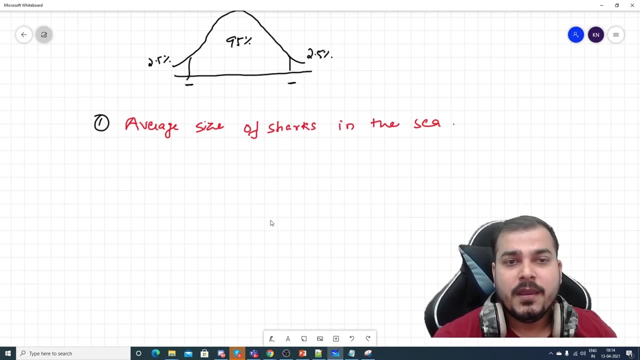 central limit theorem. one can be done with the confidence intervals right, with population standard division, without population standard division. so let's first of all focus on this and central limit theorem will not be discussing over here. we'll just try to do with the confidence interval. probably in the upcoming videos i'll try to create this, okay. so first of all, uh suppose, 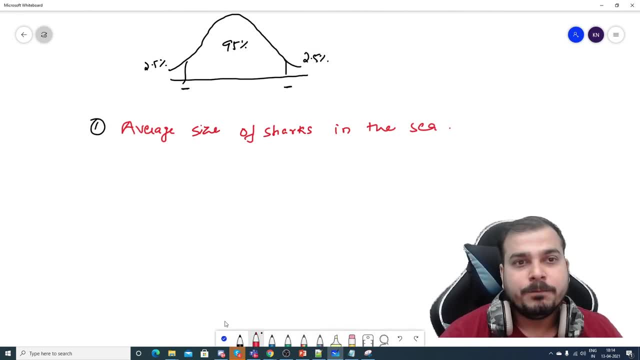 if i consider solving this with the help of, uh, probably with the help of confidence interval, where population standard deviation is given. suppose, consider that my population standard deviation is basically given as 100. okay, now, what i do is that, in order to solve this problem with the help of, 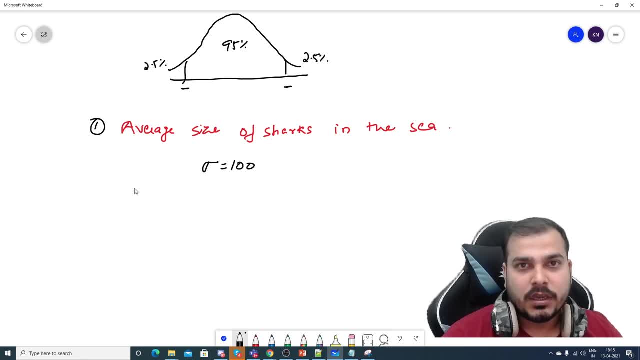 confidence interval. i will definitely take a sample, okay, sample, i can basically write it as small n, probably, i'll say, and usually the sample size that i'll try to prefer, uh, probably greater than 30 or greater or equal to 30, okay, and then, um, what i will do is that, going forward, uh, this sample. 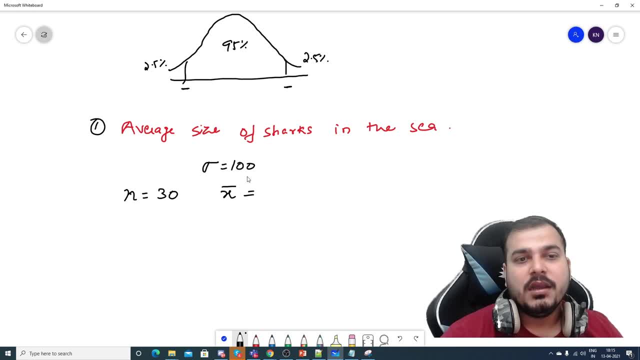 i'm trying to calculate, i will actually get x, x bar. this x bar will be probably- just consider that it is 500.. i'm just taking it as an example. the average mean size, uh, probably in centimeters, is somewhere around 500. okay, now i have all this particular information. now let's see that how. 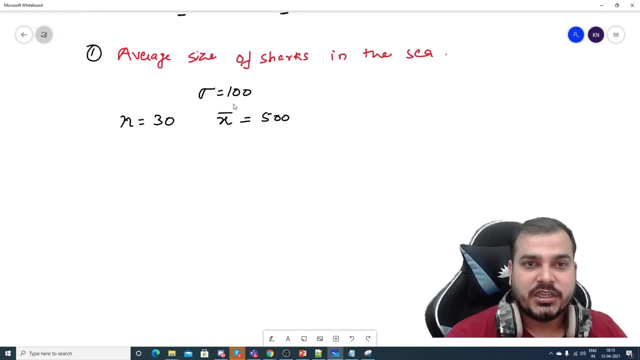 we can define the confidence interval when the population standard deviation is given. so when the population standard deviation is basically given, usually what happens is that because see he, the interviewer, has told that you can assume some of the things. okay, so the confidence interval is basically given by the formula: one is point estimate. 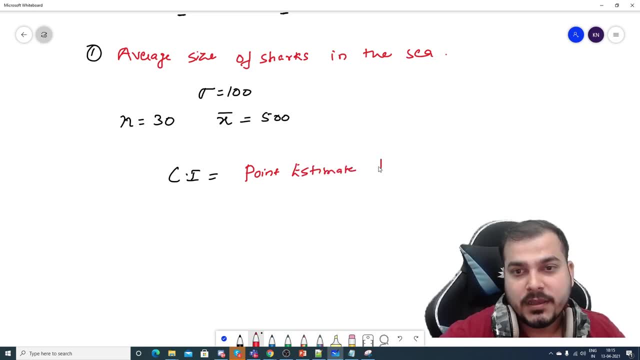 point estimate plus or minus. there is something called as margin error. okay, point estimate plus or minus margin error. this plus or minus margin error will basically- and and for this particular question i may also consider that i am taking 95 confidence interval- 95 confidence interval basically means: 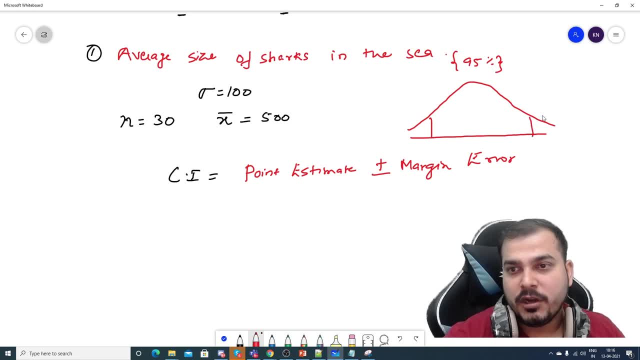 this will be a two-tail test, okay, so this is my 2.5, this is my 2.5, which is my extreme end, and this will basically be by 95. so i should basically be able to find out this specific range- uh, where- which will actually help us to tell us the confidence interval of the mean of the. 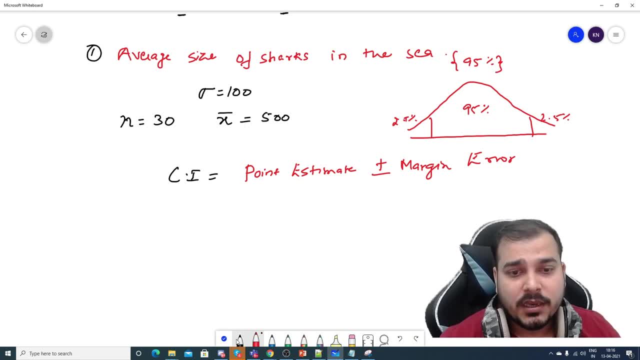 population mean. that may range. okay, point estimate over here is basically my x bar, which is my, which is my sample mean. okay, sample me, then i can write plus or minus. okay, this margin error is usually given. now, in this particular scenario, whenever your population standard deviation is given, you have to use z test. so this z will be given by alpha, by 2.. now this alpha 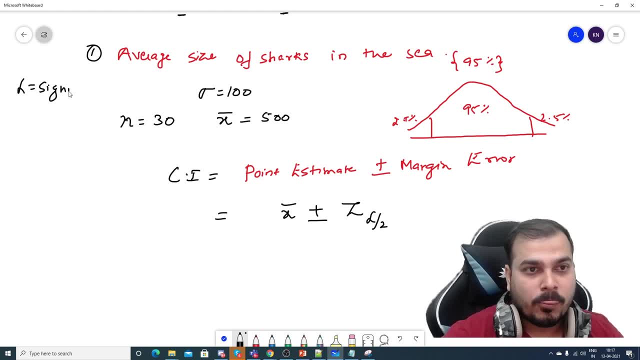 alpha is basically my significance value. significance value now, in this particular scenario where i have 95 percent confidence interval, my alpha will be nothing, but it will be just like this 2.5 and this 2.5. so, in short, this 2.5 plus 2.5 is 5 percent now if i raise. 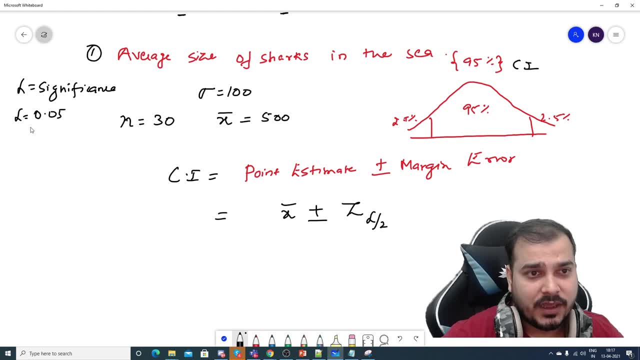 i really want to give. remove this percentage, it will be like 0.05, right? so this alpha will actually be my 0.05, which we also say as p value. it should be less than p value. less than 0.05 basically means that it is actually the. the values are present in the extreme end, extreme tail end. so 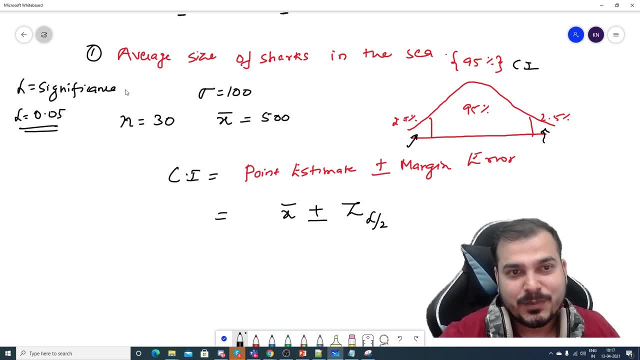 this is my tail end right. so, similarly, i'm taking this specific significance value- okay, because 95 confidence interval is given. so this alpha will be replaced by 0.052, and then i have my standard deviation divided by root n. so this is the exact formula in order to find out the confidence. 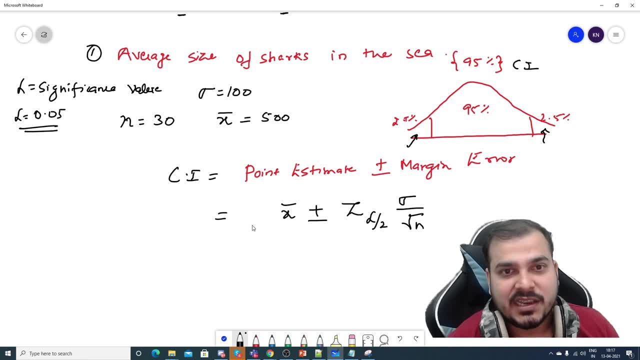 interval when your population standard deviation is basically given. and here now what i can do is that i can put down this particular value and it will have plus or minus z, and this alpha will be nothing but 0.05 divided by 2.. this standard deviation is nothing but 100 divided by root n. 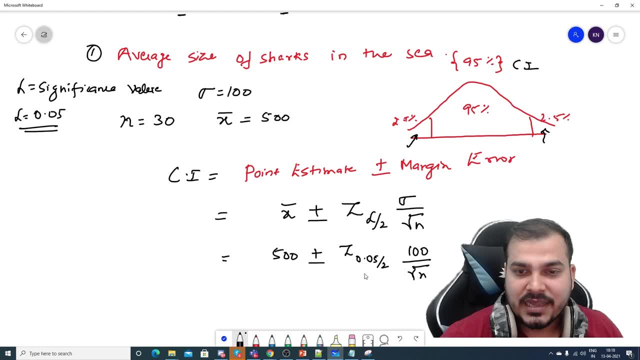 okay, and then i can still now. now the thing is that this z 0.05 divided by 2 becomes- uh, i can basically write it as z 0.025. right now, this is z 0.025. how do i calculate? i have to basically use something called as z table, so let me just open a browser and search. 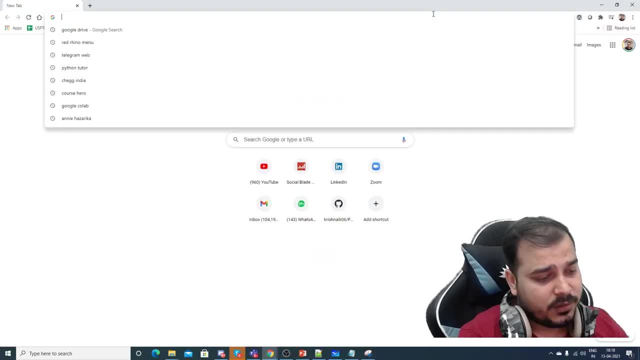 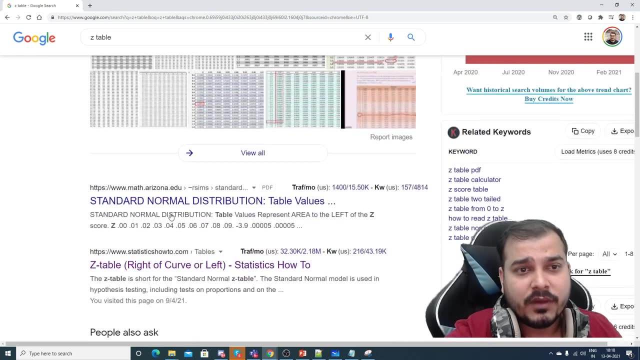 for the z table. okay, so here is my z table. so i'll write z table. okay, i'll just google it and here is my. let's see where, where my z table is, and you can select any table that you want. so i'll go and select this z table now inside. 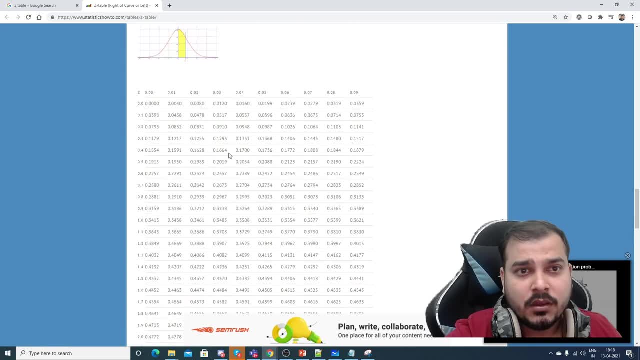 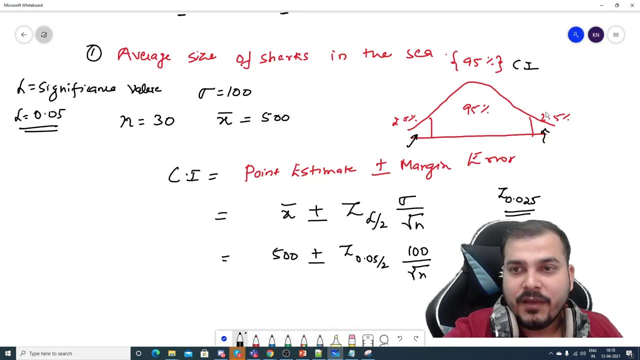 my z table. i have lot of values, uh, so see, uh, with respect to the z table. now, first of all, i need to find out two things. guys see over here, whenever i have this z 0.025 right, when i have 0.025 this. 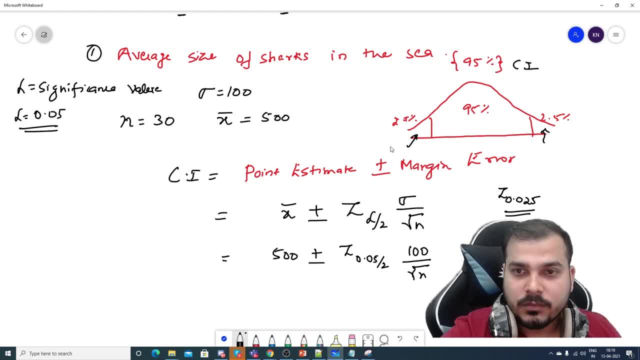 basically means that i need to compute- uh, i can basically take this entire area as one. okay, because this is anyhow two tail test, right? so 2.5, 2.5 will be over here now in order to find out the area like this: 2.5 is basically present. i can basically write: z is equal to. i can just define this as: 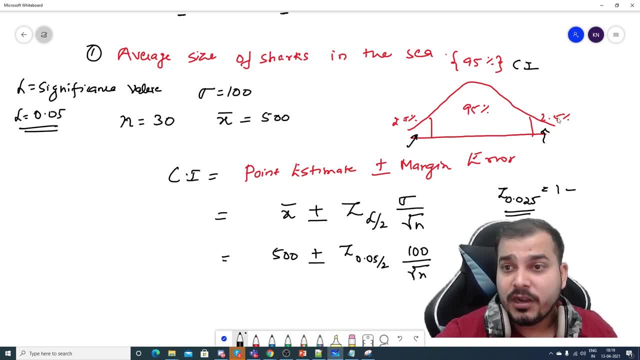 1 minus, because 1 is the entire area minus 2.5 percent, it is nothing but 0.025, right? so if i try to calculate this, it will be 0.975. i guess 0.975. now i need to find out this 0.975 in my z table. 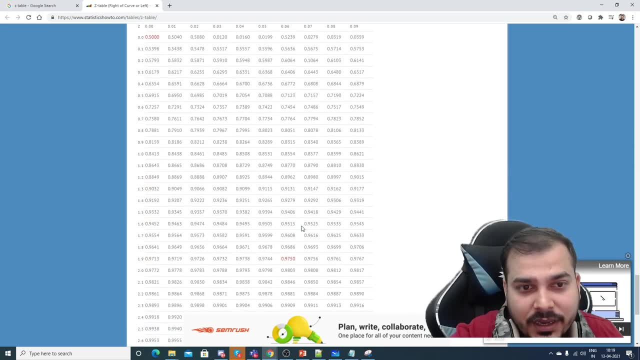 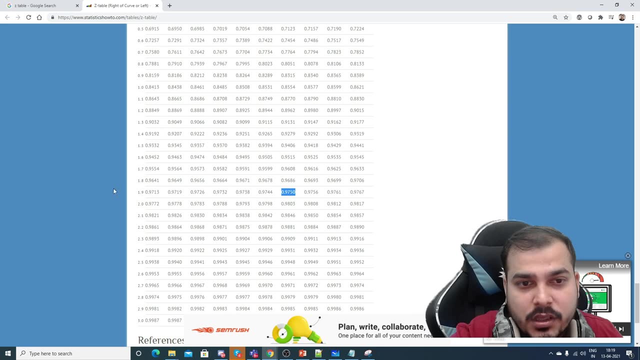 so 0.975 in my z table will give us what value let's see. so if i go over here, 0.975, 0, so here you can see 0.9750. i have to see this, guys. i will just zoom in. so here i have 0.9750. 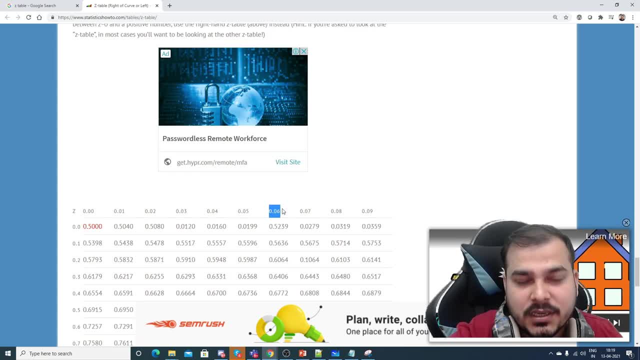 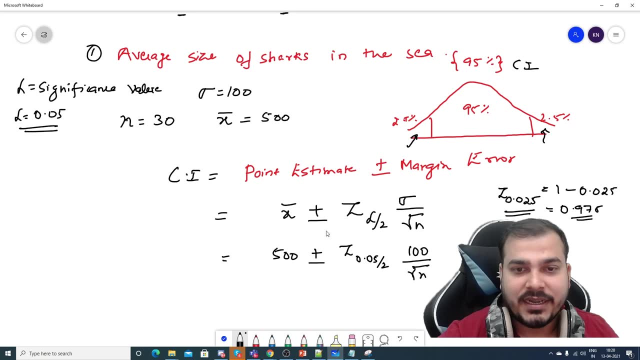 this is 1.9 and if i go on the top it is 0.06, so it will be 1.96. okay, so 1.96 should be this particular value based on the z table. let me write it clearly and properly. so this z: 0.05. 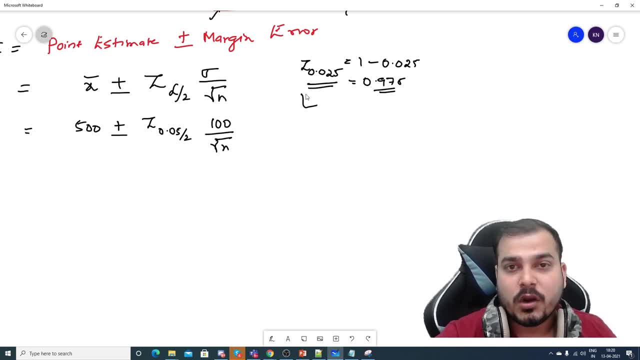 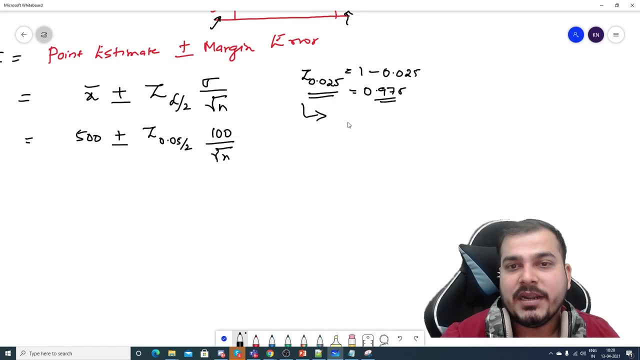 uh, when i'm trying to find out this point, zero nine five, seven five according to the z table- it is actually giving us what value it is basically giving us. uh, you can see over here 1.96. so here you can see, 1.96 will be my. 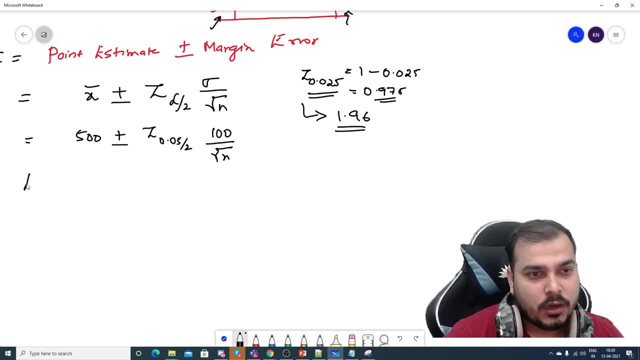 value with respect to this z value. now, here i will be calculating my first of all, my lower limit. so my lower limit will be 500 minus z. see minus and plus are there. first of all. i'll try to calculate minus. this are z 0.05, which is uh divided by two, it is nothing but z. 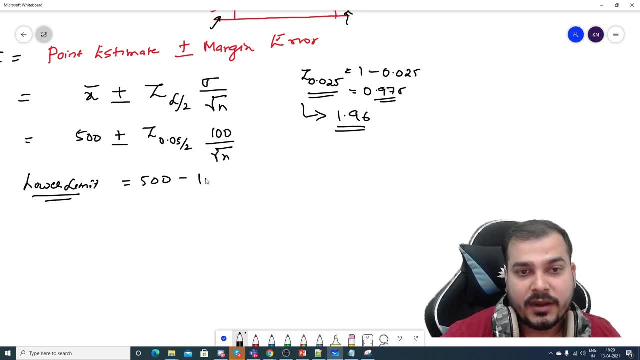 0.05. it is nothing but 1.96. so this i'll write it as 1.96 multiplied by 100 divided by root of 30. okay, so this will basically be my lower limit and this will be my higher limit. so the higher limit. 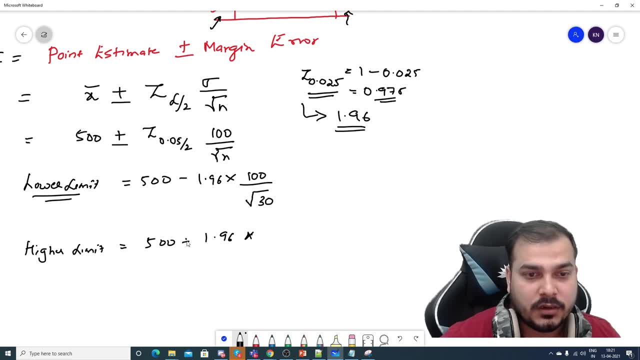 says 500 minus 1.96. sorry, it will be plus 100, divided by root 30. okay, now what i can do. i can basically calculate uh with the help of scientific calculator. just let me open scientific calculator just to find out, like uh, quickly how. so it is 100. um, you want to check it out? i can just show you. 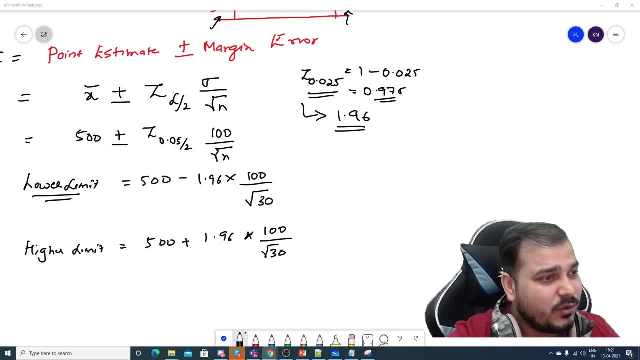 but let me just quickly do it for you so that you don't have to worry, because so, multiplied by 1.96 is equal to uh minus 500, okay, minus 5. so this value is exactly: is somewhere around 386, uh, approximately equal to 386, and. 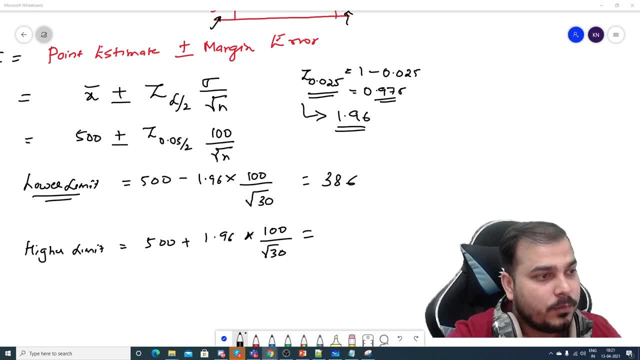 if i try to calculate the same value, just let me show plus 500, plus 500, equal to plus 500. okay, so this particular value that i'm getting is somewhere around 613.. now, this is my lower limit, this is my higher limit. now, what this particular range gives us, this is: 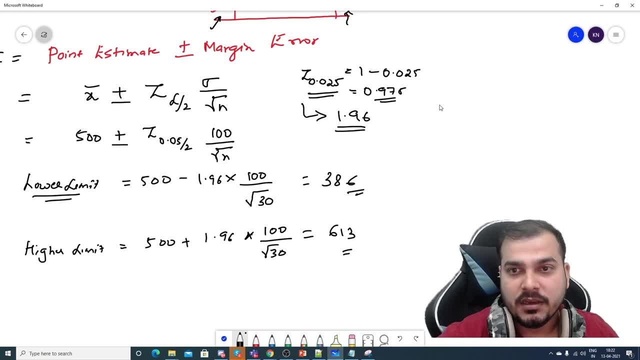 my main, what's our range? and this is essentially my confidence interval. it says that my population mean, that is mu, okay, i will be having somewhere around 95 percent confidence interval that my population mean will be falling between 386 to 613. this is the information that i have to give my 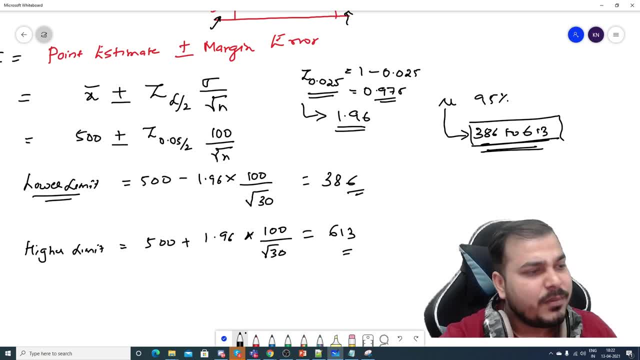 interviewer who is basically asking this particular question, right? so over here you could see that we are able to quickly find out that what will be the range- okay, what will be the range of this or times range, because we can just check and viz what we say for a contribute we'll give. so we will do three. 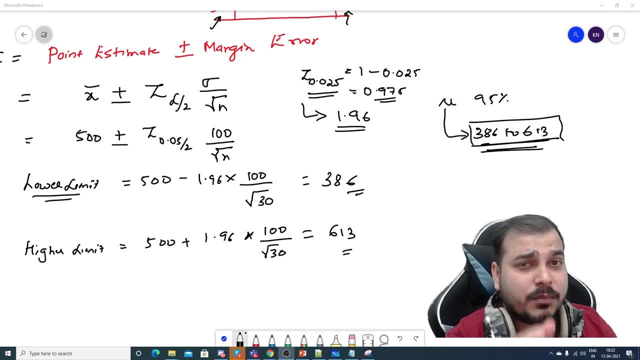 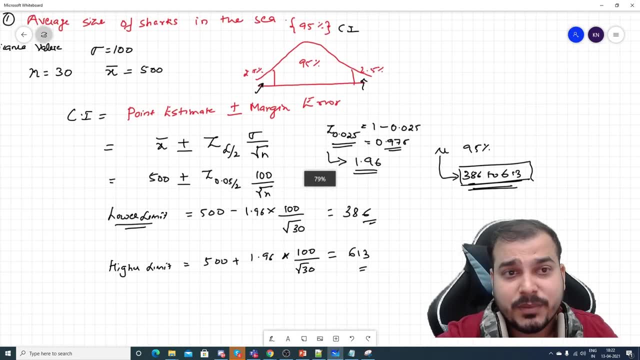 the population mean, based on our sample mean and the population standard deviation. now, this was the information. this is what the interview question was basically asked. right, because this was the question that was asked by my subscriber. how do i find out the average size of the shark in the sea?